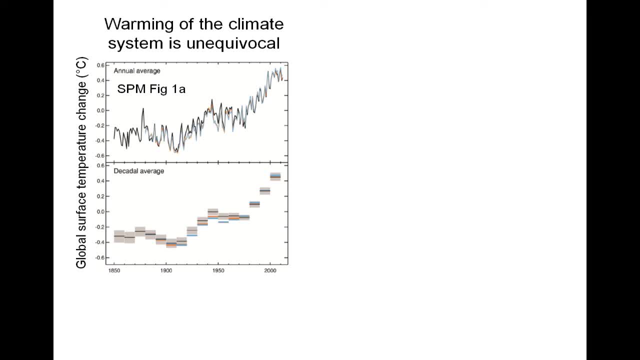 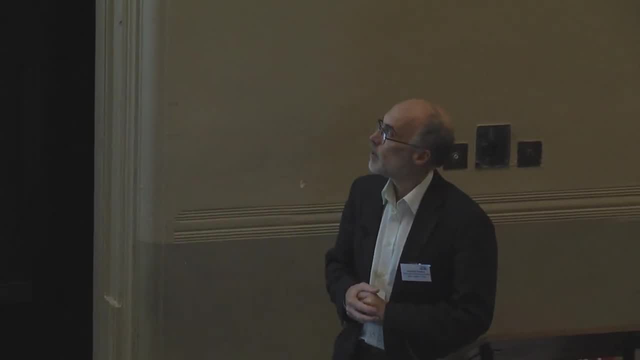 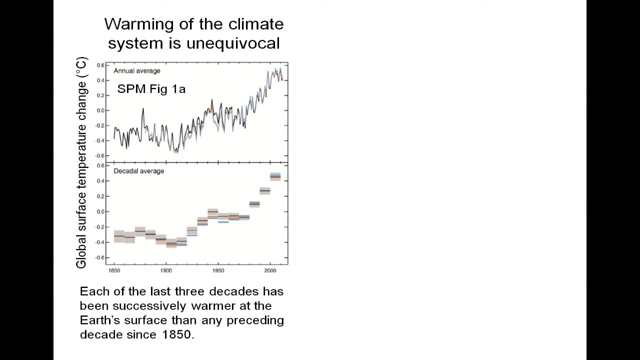 conclusion, in particular, ocean warming, as Annie has shown us, reduction of ice on land, as Jonathan has shown us, and the global mean temperature time series, updated to 2012, is shown here. If you fit a trend from the latter part of the 19th century to now and use that to work out how much the temperature has gone up, 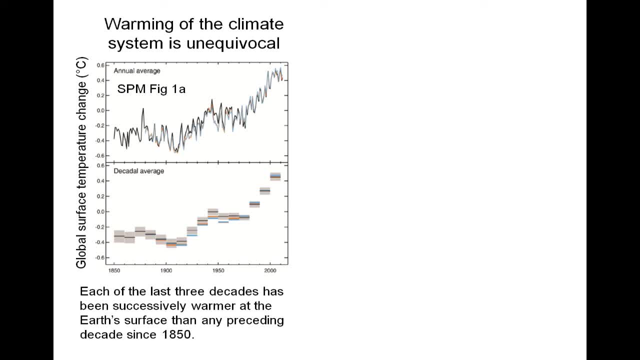 the answer is about 0.85% degrees. The lower graph shows you decadal means, which of course gets rid a lot of the variability and points to the striking conclusion that each of the last three decades, that's calendar decades, has been successively warmer at. 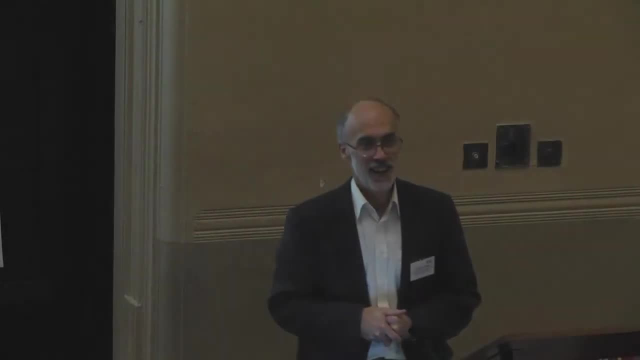 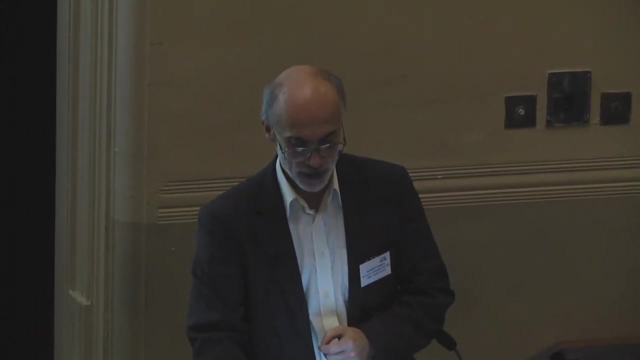 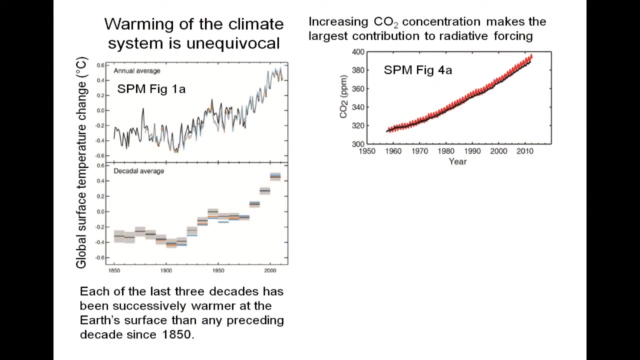 the Earth's surface than any of the preceding decades, and that is quite clear, I think. Now we know, of course, on physical grounds, that we would expect an increase in greenhouse gases in the atmosphere to warm up the Earth's system, and we expect that CO2 concentration, from calculations, has made the largest contribution to that. 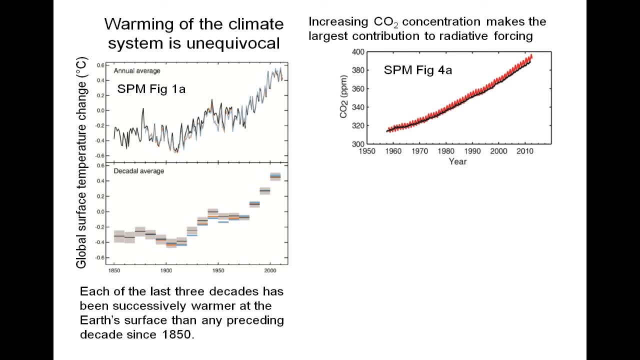 radiative forcing. We know for sure that it has been going up in the instrumental period since the 1950s, during which it's been directly measured, and we know from ice cores that it has been going up on longer time scales and now stands at a. 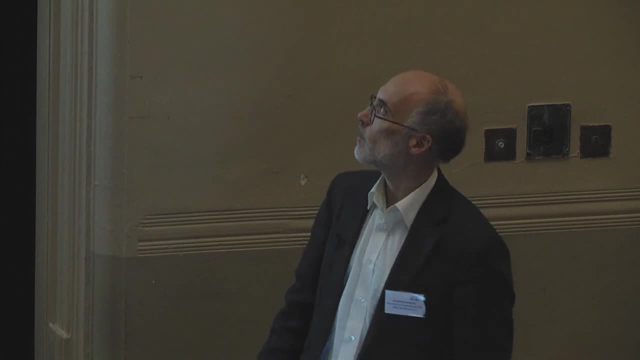 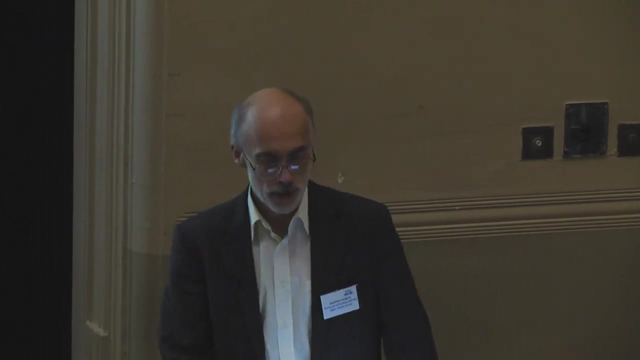 level that hasn't been reached for at least 800,000 years. that is the length of the ice core records Since the Industrial Revolution. we can explain the amount by which CO2 has gone up in the atmosphere, and it's about two-thirds due to. 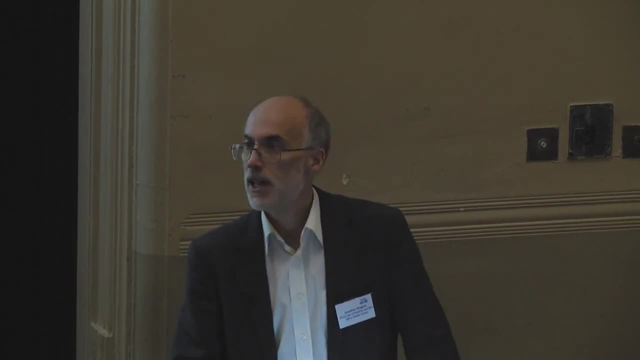 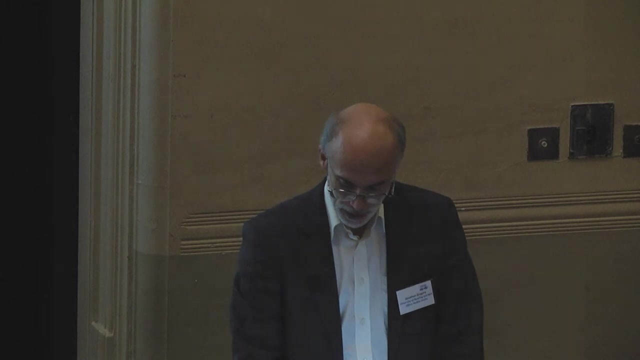 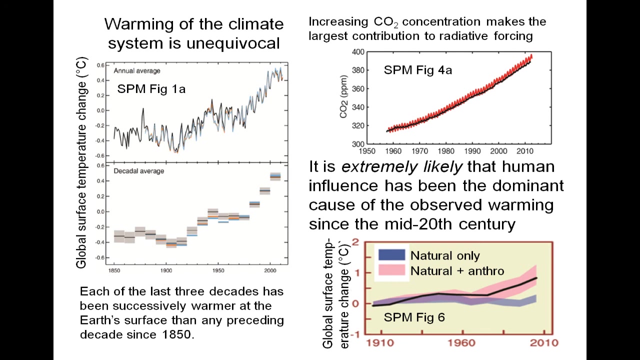 fossil fuel combustion, one-third due to land use change, but now it's about ten to one in favor of fossil fuel combustion at the present time And, as a result of that, by putting the CO2 concentration and the concentrations of other greenhouse gases and anthropogenic agents into climate models, it is 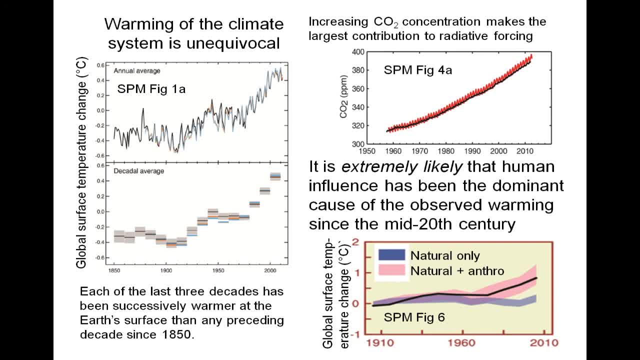 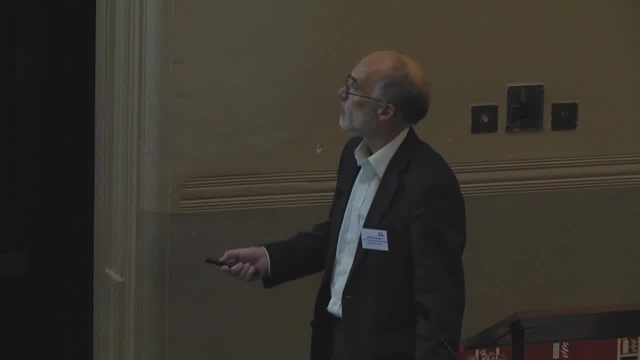 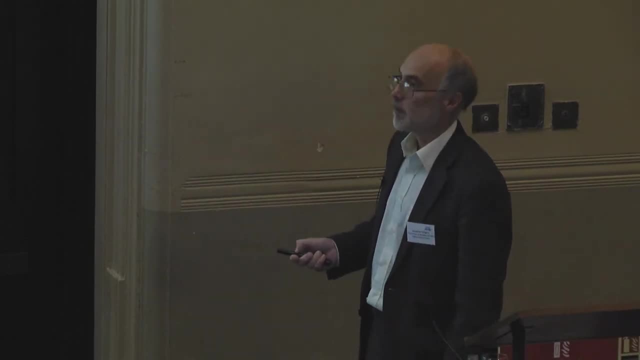 possible to reach the conclusion that it is extremely likely that human influence has been the dominant cause of observed warming since the mid 20th century, And that's the way it is. Thank you That is based on comparison such as this one, where the simulated model mean global. 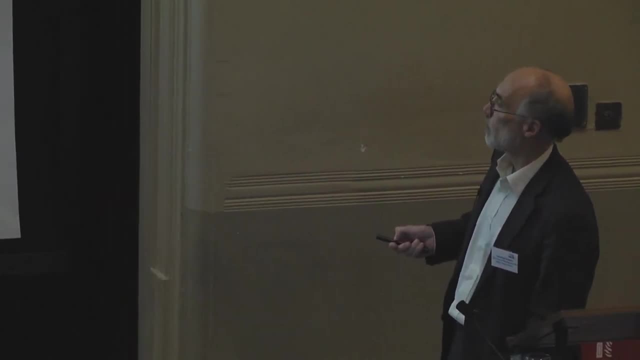 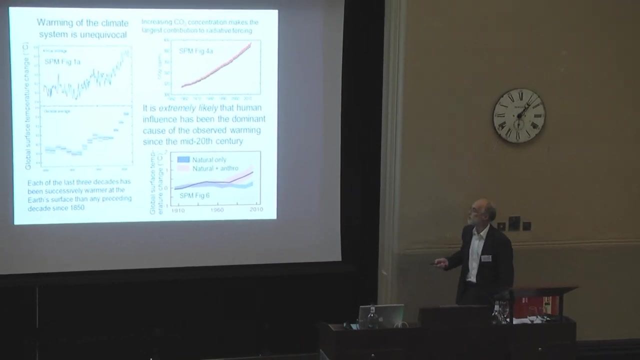 temperature time series, which is a pink. well, this is the model range. the pink band agrees very well with the observed change, Whereas if you omit the anthropogenic forcings and you just have natural forcings, then you have a global warming, And if you omit the anthropogenic forcings, that is principally. 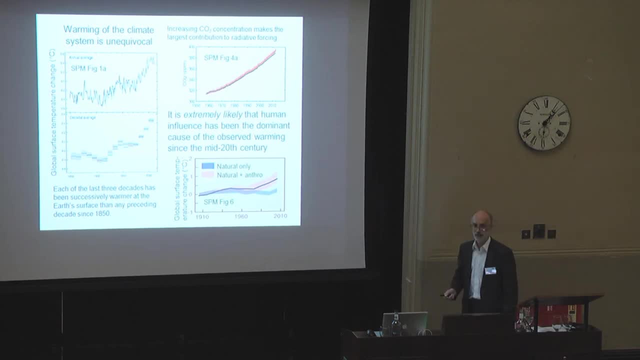 volcanic eruptions and solar irradiance changes, you don't get that recent increasing trend. So you're familiar with all those conclusions. Now, a global mean sea level rise is also sometimes cited as evidence of global warming, And to some extent it is, but it's not quite as simple as that. On the long term of 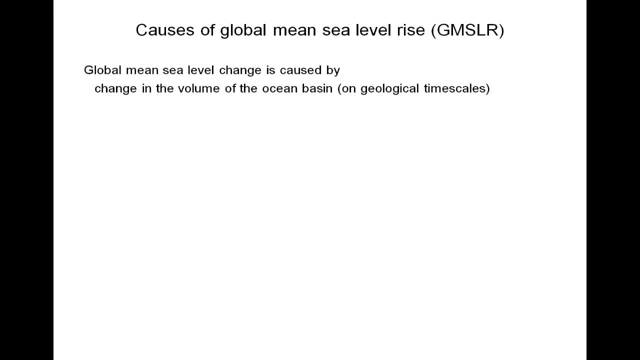 course, geological time scales, global mean sea level rise is caused by change in the volume of the ocean basin, amongst other effects. But if we consider only climate change time scales- centuries or millennia- what we are concerned about with global mean sea level rise is a change in the volume of water in the ocean, And that is caused by 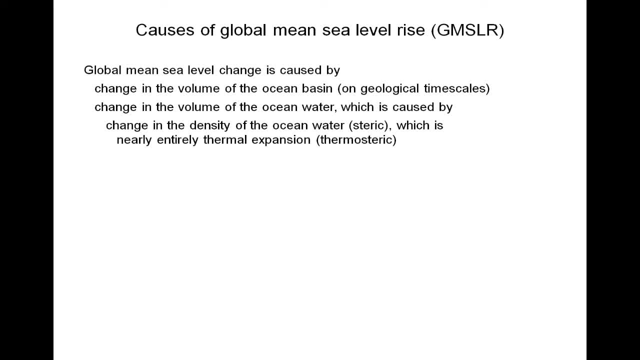 change in the density of the ocean water, as has been discussed by Annie, who showed the budget previously, which is nearly entirely thermal. expansion due to warming, and changes in the mass of the ocean due to water going into the ocean, which is currently in the form. 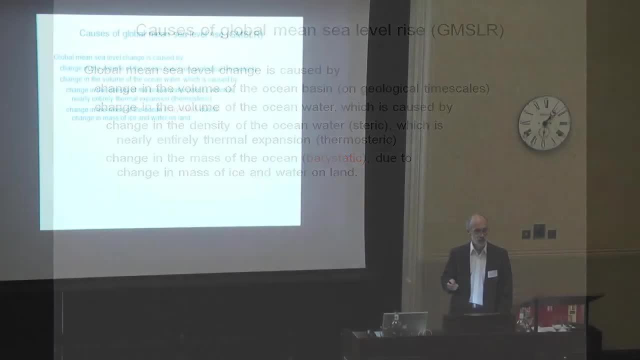 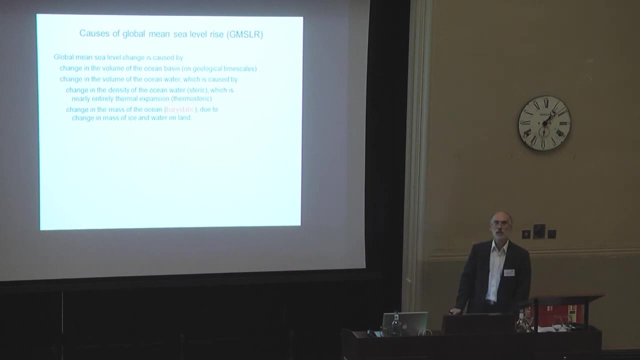 of mass or water on land. I would like to make an advertisement for the new word baristatic, which may or may not catch on, but this word is proposed to mean the contribution that comes from adding mass to the ocean. The change in global mean sea level comes from adding. 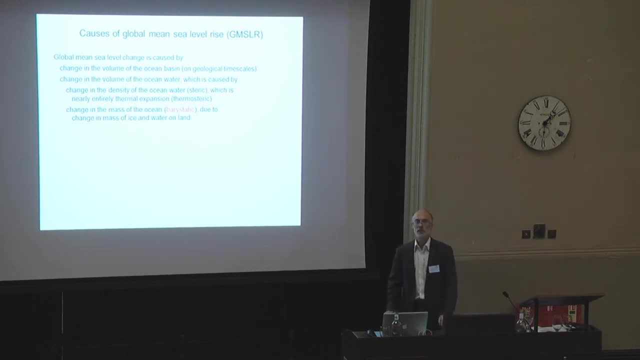 mass to the ocean. Of course you could call this the mass term, but in some contexts that's confusing, because the mass term could mean the change in local sea level caused by the modification to the geoid. Another word that has been used for this is eustatic, but that's. 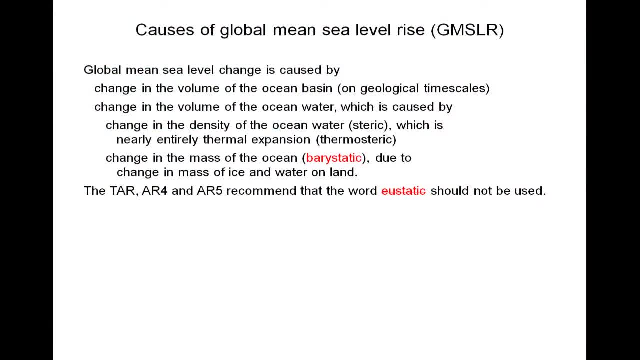 confusing too, because the original meaning of eustatic is global, mean sea level change. so that means it has two meanings which have been used. One is eustatic and the other is global, mean sea level change. So that means it has two meanings which have been used. 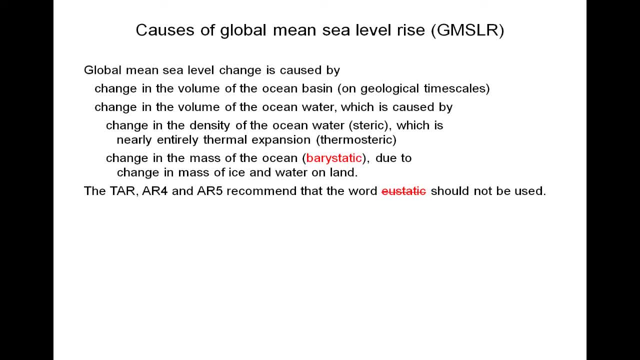 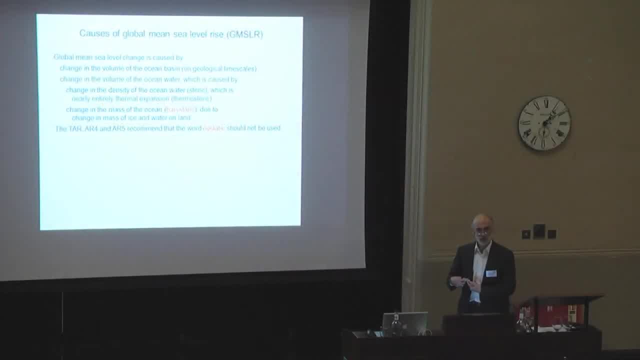 but they're not consistent and for that reason the last three assessment reports have all recommended the word eustatic should not be used, So this word, baristatic, is proposed as a possible alternative, if you would like to use it. It's a newly invented word that. 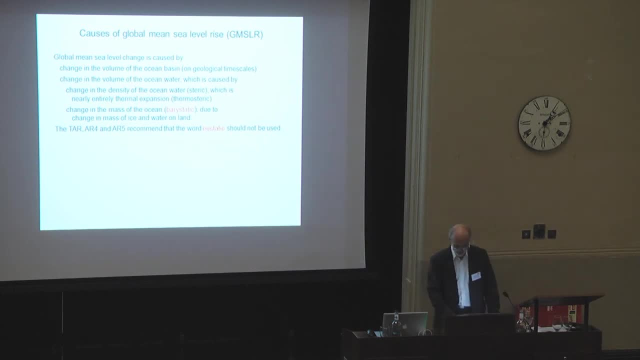 hasn't previously been used, except in Star Trek, where it means something different. Now I'd like to talk about the contributions to global mean sea level rise and how we reach our assessment of confidence in the projections of global mean sea level change. One of the things that carries a lot of pride is this high confidence that we make in the 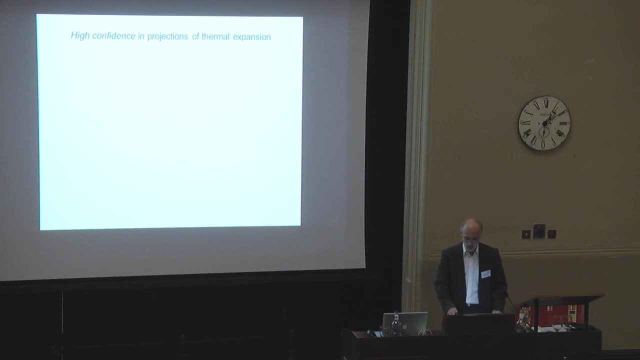 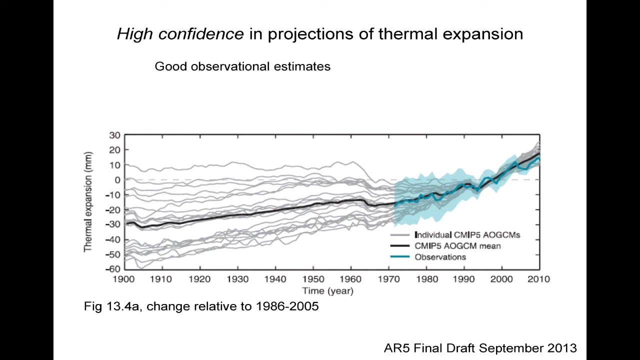 AR5. We've got how I confidence in the projections of thermal expansion and this is because we now have good observationally based estimates of thermal expansion, as Annie has shown us. that is shown here as the blue chains band and the solid blue line which 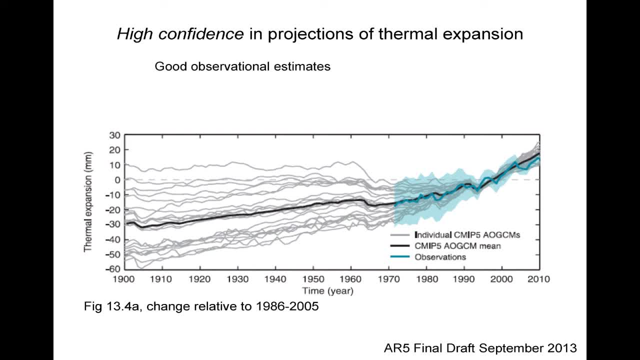 is the mean in the middle. So this is a calculation from an observed ocean 3D temperature something and this record has improved a lot since the AR4 because of the identification and correction. EE technically have well-developed thermal sense of correction of some observational errors, so we've got more confidence in that than we used to have. 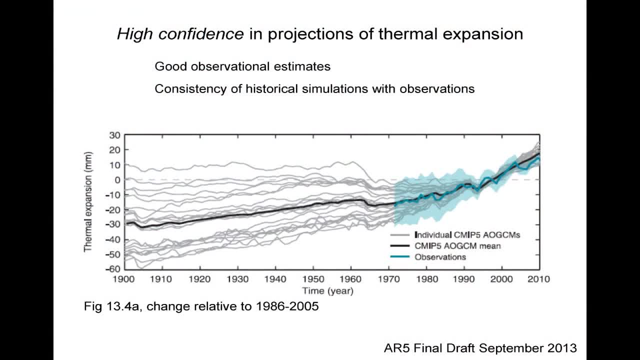 then we also have the consistency of historical simulations with GCMs, with the observations. so these grey lines here are individual GCMs and the solid black line is the mean of GCMs. and you can see there's a very good agreement between the GCM ensemble mean and the historical. 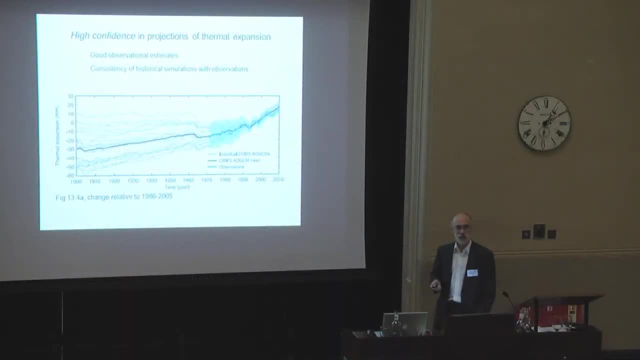 record because the GCMs have been forced with anthropogenic and natural forcings. this gives us evidence that the warming of the ocean is at least partly anthropogenic, but there is also a natural influence which can be seen from the dips in the black lines and 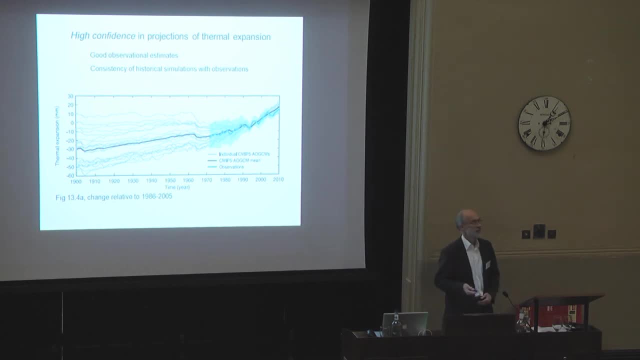 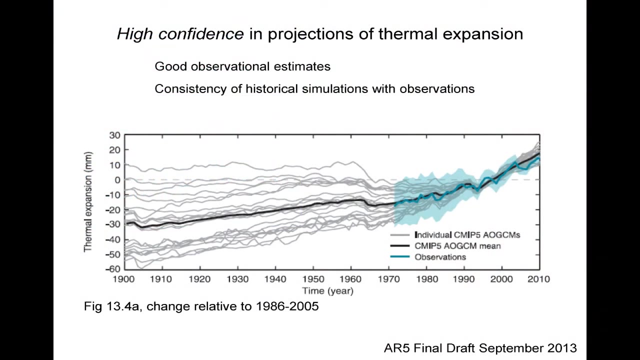 that's when a volcano erupts that temporarily cools the earth system. so we expect to see that signature out there as well, but clearly it's not dominant. there's more variability in the in the observed record than there is in the black line, because the black line is a mean. 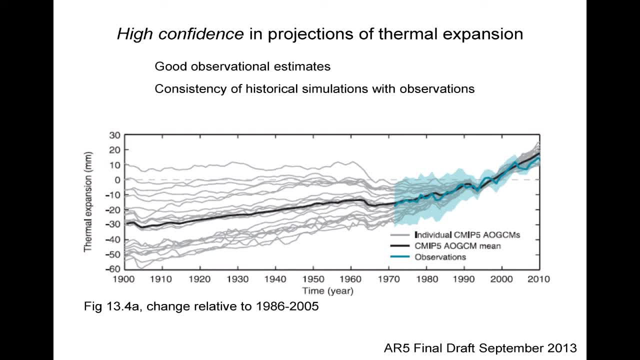 over many GCMs, so internal variability, such as ENSO effects, tend to be averaged out. and thirdly, we have, overall, a better understanding of the earth energy budget, which means that we can demonstrate a consistency between our estimates of radiative forcing, climate sensitivity and the amount of heat that is observed to being stored in the earth system. 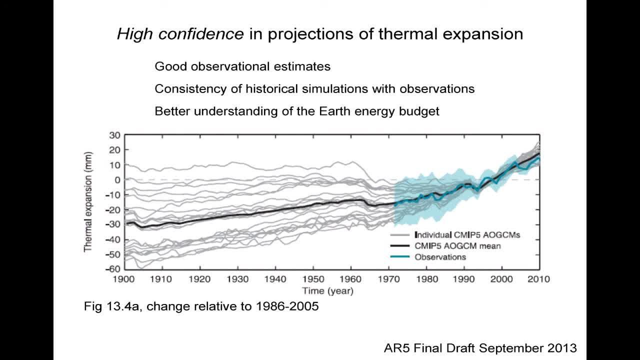 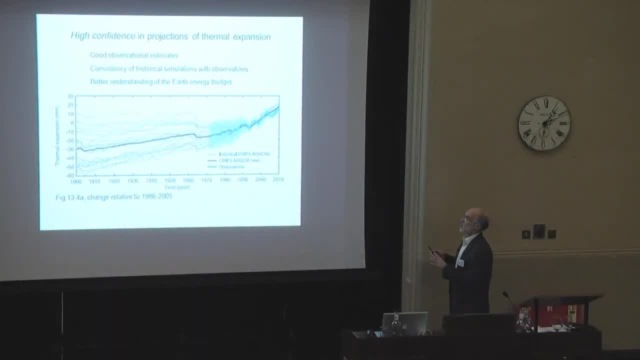 and because this kind of this budget is relatively is well closed within uncertainties, that leads us to believe we have some idea about what's going on. so these, these strands of evidence mean that we have high confidence in our ability to project thermal expansion using GCM: projections of ocean temperature change. 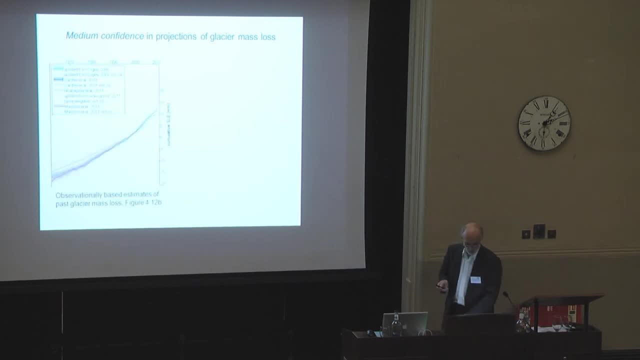 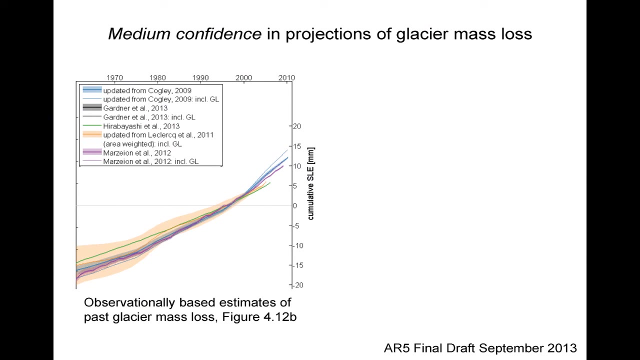 we've got medium confidence in projections of glacier mass loss. again, we've got records of glacier mass loss- Jonathan has talked about this already- going back several decades, and there is a consistency of historical simulations with observations for this too. so this, this figure, actually comes from chapter four and the important point is the. 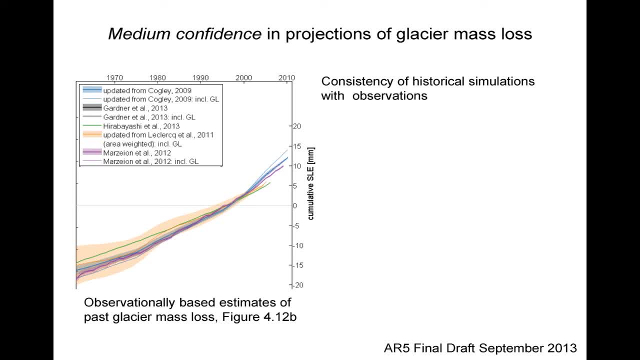 purple line of Marzayan et al is actually a model of a version of the Marzayan et al, which is actually an artificial model, whereas the other ones are glaciological measurements based on glaciological measurements, showing an agreement there. and this gives us confidence, because the model of Ben Marzayan is the same kind of model. 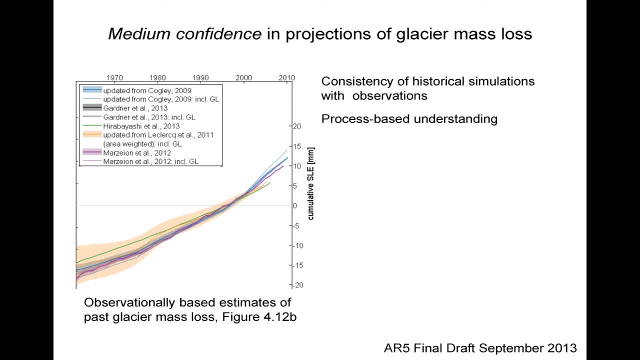 as we use to make projections, and those models have a process founded on process based understanding of what are the influences on on glacier mass balance, although they are simplified for dealing with the total ensemble of the world's glaciers. confidence, but we assess our confidence only as medium because, as Jonathan's mentioned, the set 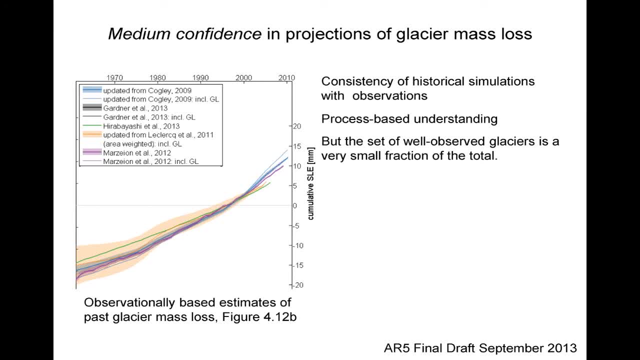 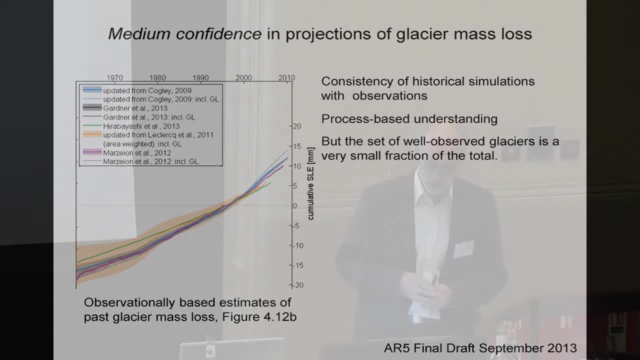 of well-observed glaciers on which the observations are based and the models are calibrated is a very small fraction of the total number of glaciers in the world. so because a sort of extrapolation is involved, we can't be entirely happy about that. and then, going to ice sheets, I have a figure here. 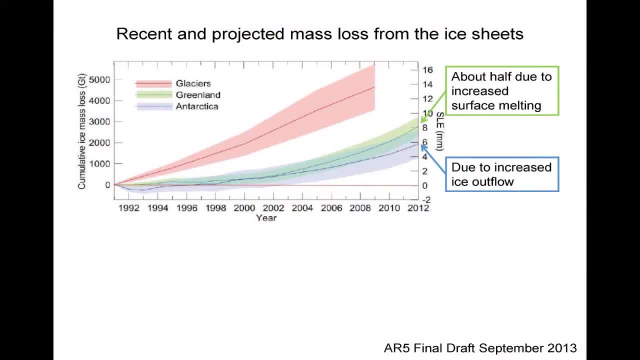 which you've really seen twice before. we all have a different thing to say about it. so we know- thinking first about greenland- from the comparison of different methods of measurement of the change in mass of the green and ice sheet that about half the increased mass loss is due to increased 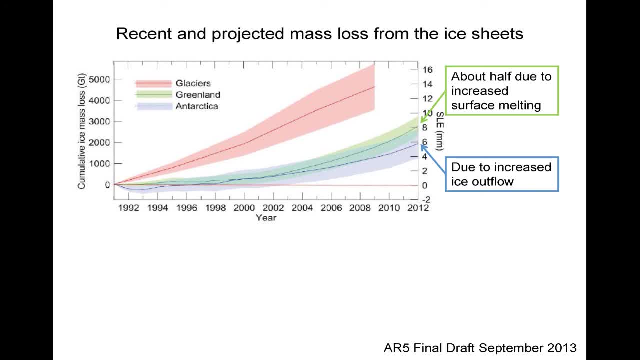 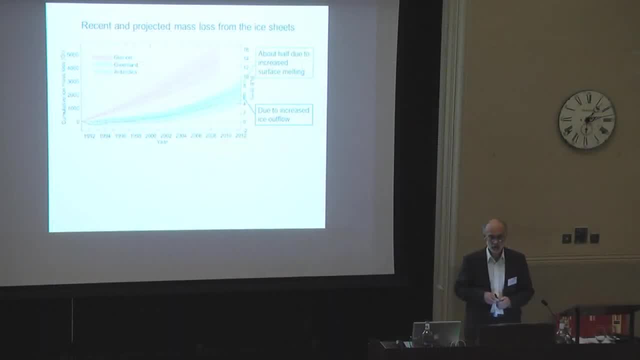 surface melting over recent years, meaning the other half must be coming from increased ice discharge into the ocean. now the the the modeling of surface melting is done with high resolution climate models, typically of the same kind as we use to make projections. therefore, the agreement of observations with models for the past gives us the same kind of results as we used to make. 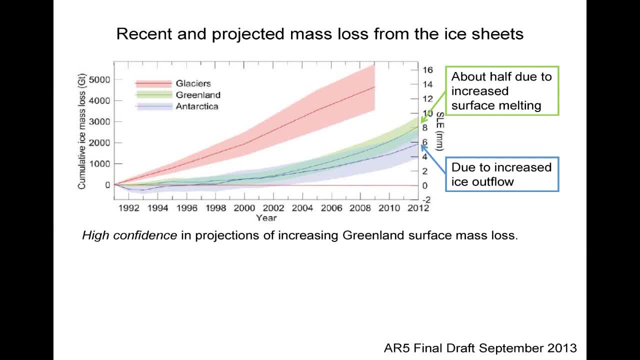 and that gives us confidence in our projections of increasing greenland surface mass loss in the future, which is an obvious consequence of warming that will occur in greenland, leading to greater melting exceeding the expected increase in precipitation. we also expect that greenland will warm more than the global average, whereas for Antarctica we also have rcms that can give. 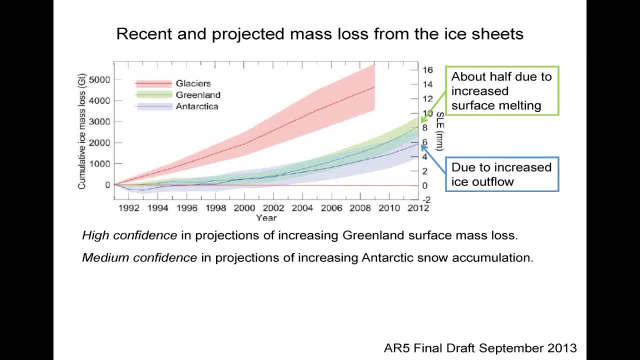 us surface mass balance which, in the case of Antarctica, is essentially precipitation, because that is snowfall, because there is practically no melting. but, as Jonathan said, the these models, when considering the past, don't show a trend in increasing antarctic snow accumulation and therefore the increasing rate of mass loss in 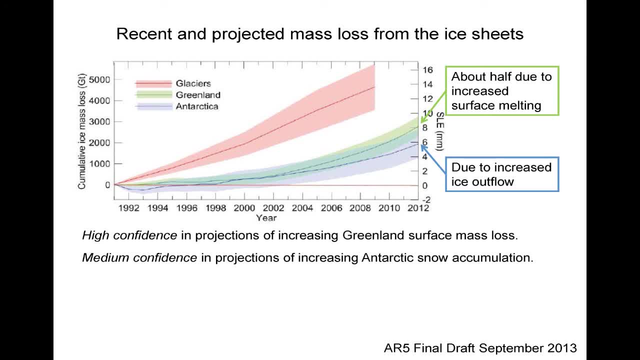 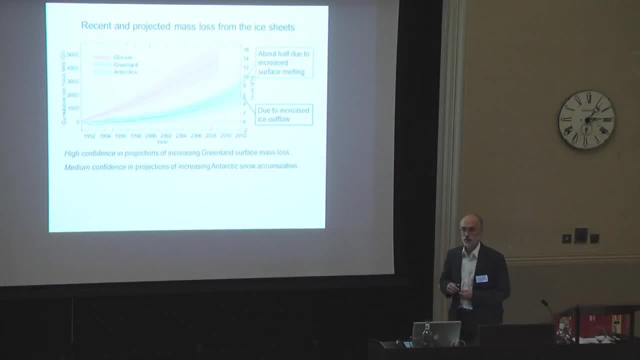 the antarctic must be entirely due to increased outflow, not due to melting, because there is not any now. all GCMs, global GCMs project, project for the future that Antarctica will warm and, consistent with that, there will be more precipitation and therefore more. 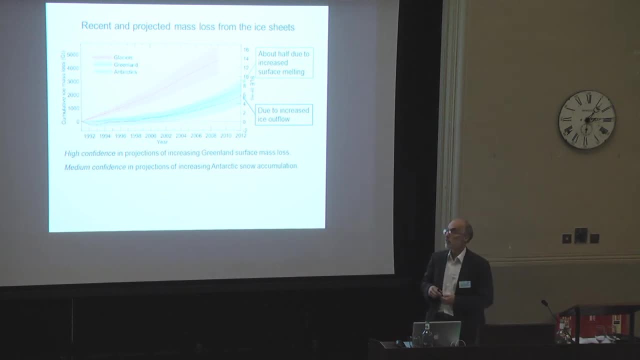 snowfall, but these trends have not been observed so far. so, despite the fact that we have good physical reasons for expecting that to happen, because it's not observed we have any medium confidence in that projection. so those are for the surface mass balance components and then for 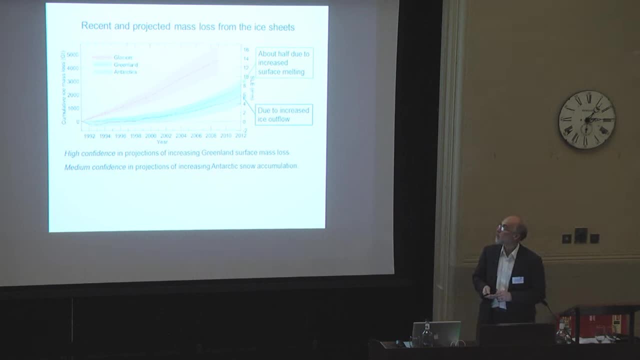 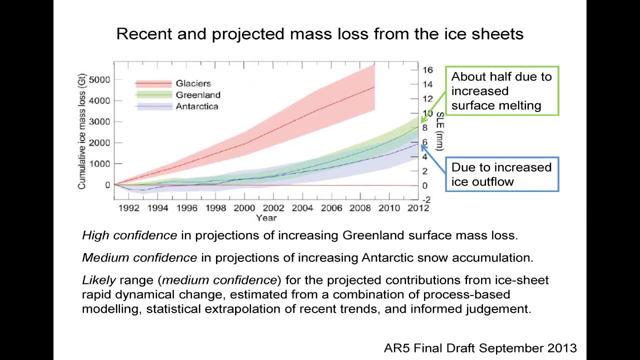 both ice sheets. we also have to deal with the more difficult question and what will happen to the ice sheet outflow in the future. and because we don't have complete deterministic, process based models of the ice sheets, we based this is assessment on the range of a range of different kinds of evidence in the literature. they are: 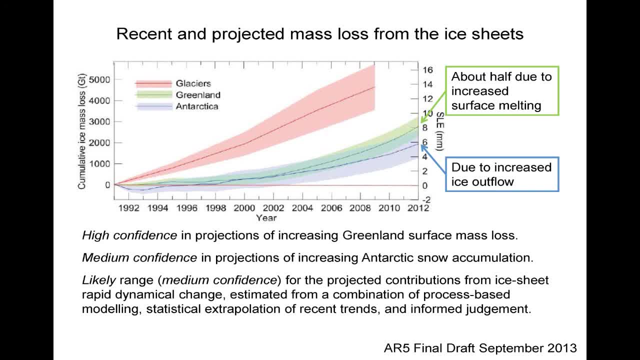 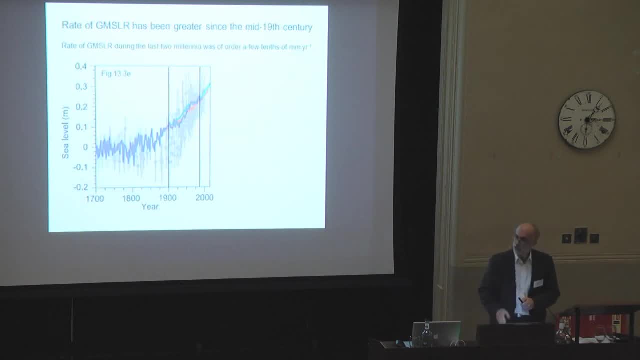 process based models for parts of the ice sheets, statistical extrapolation of recent trends and some expert judgment, and putting all these together we arrive at likely ranges for the contributions to increasing outflow from the ice sheets with medium confidence for the 21st century. so those are the components. the other source of confidence comes from whether or not we can. 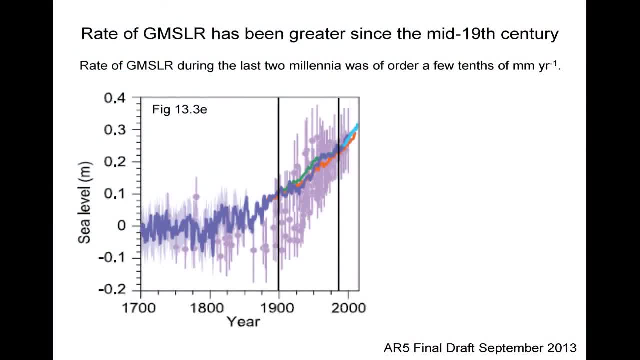 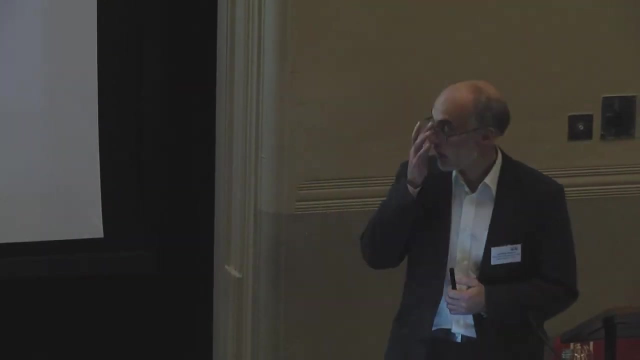 explain the total observed sea level rise. as has already been said since the in the recent policy in the last couple of thousand years, the rate of sea level rise inferred from proxy data such as particularly salt marshes. salt marsh data shown here as the light purple was small, of the order of maybe one or two tenths of a millimeter. 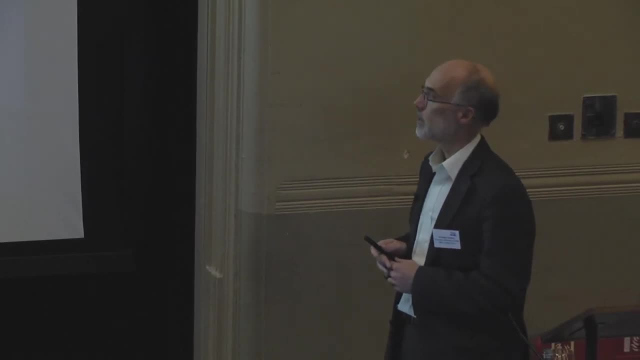 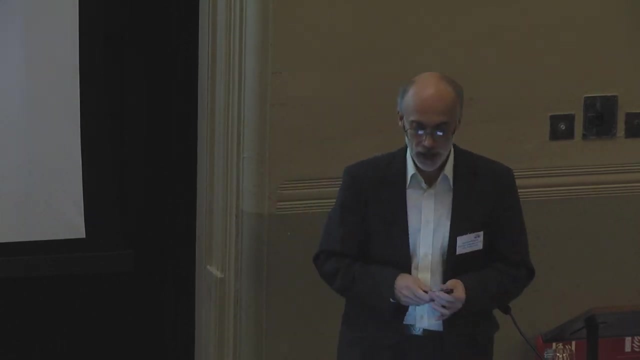 per year. but since the middle of the 19th century the rate of sea level rise or the late 19th century. sometime in the 19th century the rate of sea level rise has been substantially larger and we know from tide gauges the rate during 1981 to 1990 was about one and a half. 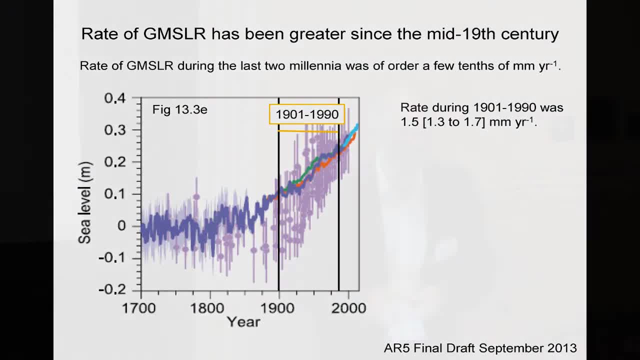 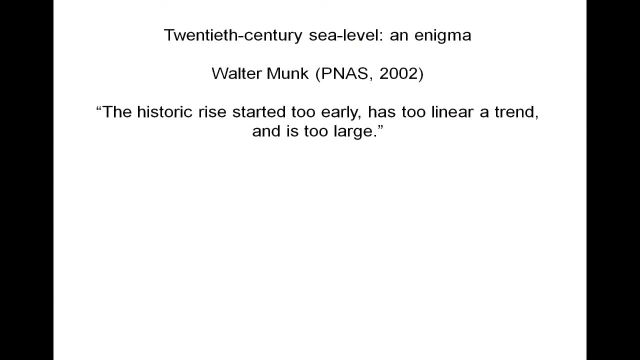 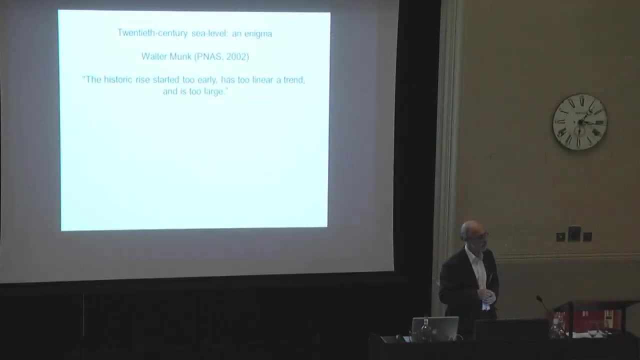 millimeters a year. in 2002, walter monk wrote a paper called 20th century sea level- an enigma, in which he complains that the historic rate of sea level rise started too early, was too linear and was too large, and this is a kind of challenge to us to explain this, and we have made progress on. 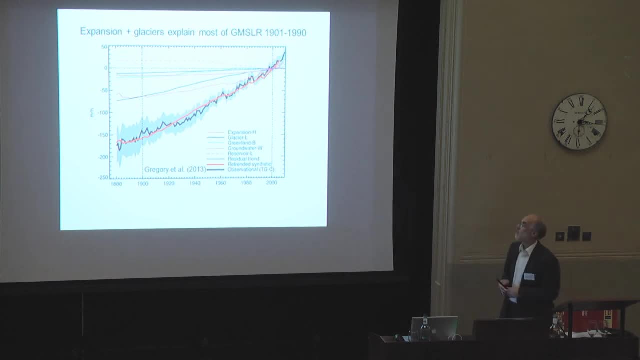 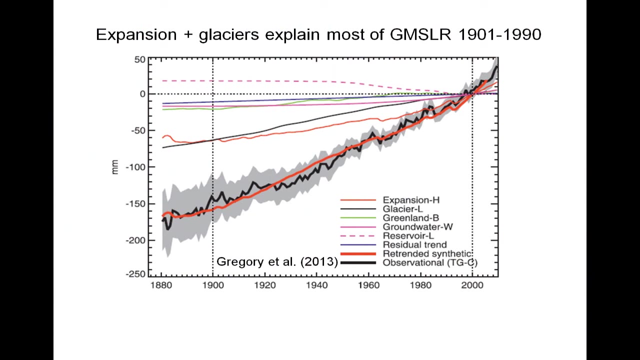 these questions in the last few years. this is a figure from a paper that was published in the newspaper, of which i wrote with many collaborators who are experts in the various parts of the budget, putting together what we now know about how we could explain sea level. this is just one. 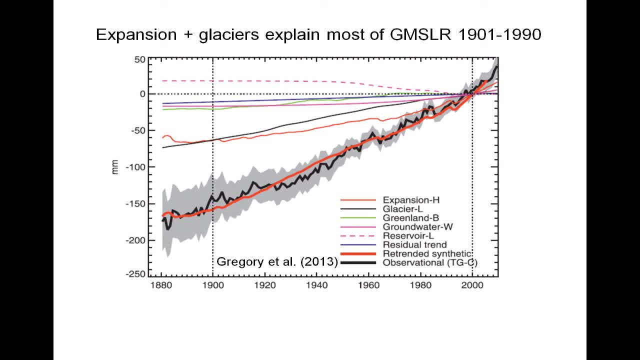 possible example. there are many possible permutations of data sets. the black line here is the observed globe, the thick black line is the observed global mean reconstruction of sea level rise by church white and the red line the solid, the thick red line that practically overrides it. is a sum of estimated contributions and you can see the number of second three line goes up here. 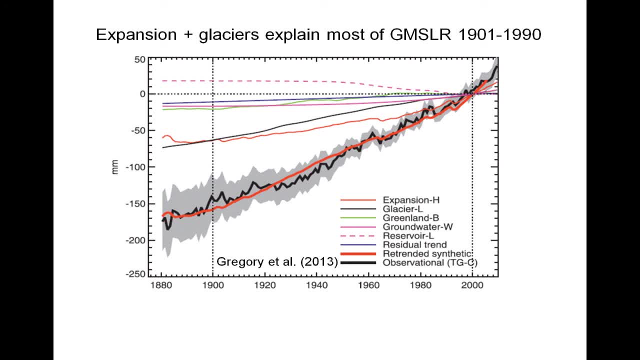 there you can see a veryố And you can see very good agreement there, leading us to think that in fact we can largely explain 20th century sea level rise. Now it is not such an enigma as it was, And the dominant contributions are the light red line- thermal expansion- and the light black line- glaciers. 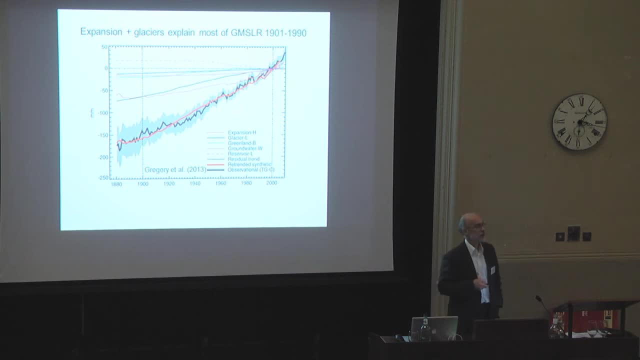 And both of those estimates are larger than previously and that's why the budget is better closed than it used to be. It's notable, I think, that the black line, the glacier contribution, is a fairly straight line, That is, the rate of mass loss by glaciers didn't increase very strongly during the 20th century. 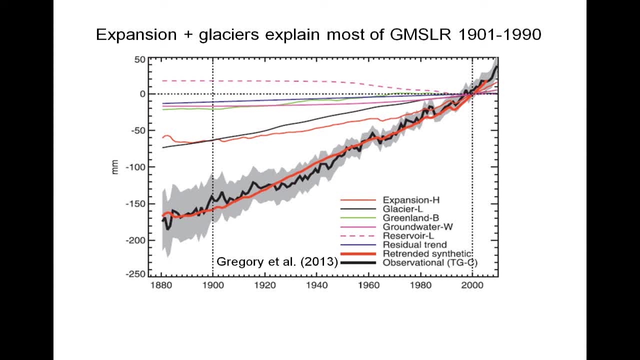 And there are two possible reasons for this that have been put forward. One is that in the early part of the 20th century there was a warming in high northern latitudes, especially in the Arctic and in Greenland, And glaciers therefore in those regions lost mass quite rapidly. 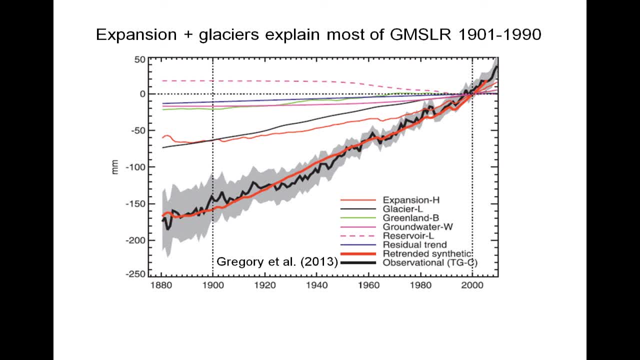 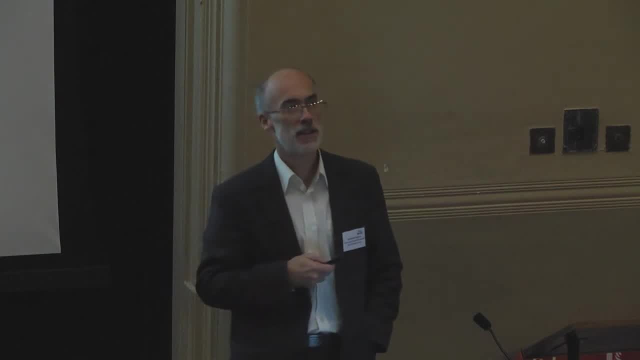 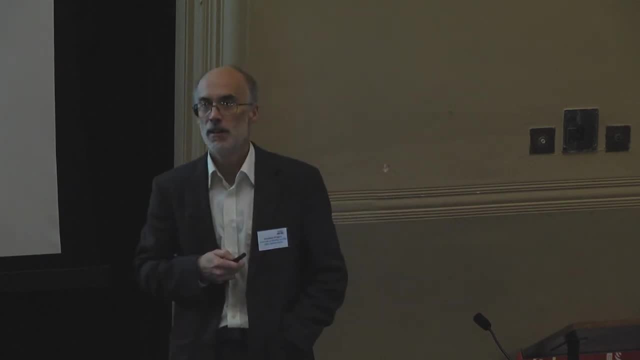 And the other reason is a general observation, that when glaciers lose mass, the parts they lose are of course the low altitude glaciers, The low altitude sensitive parts, which means their sensitivity to future mass, future temperature change is reduced. So you have a kind of compensation between the fact that the warmer it gets, the more the glaciers should be losing mass per square metre. 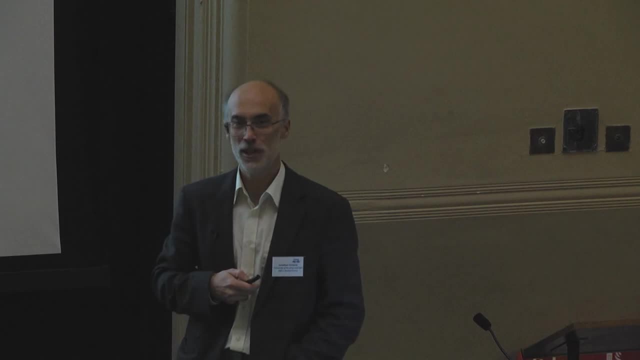 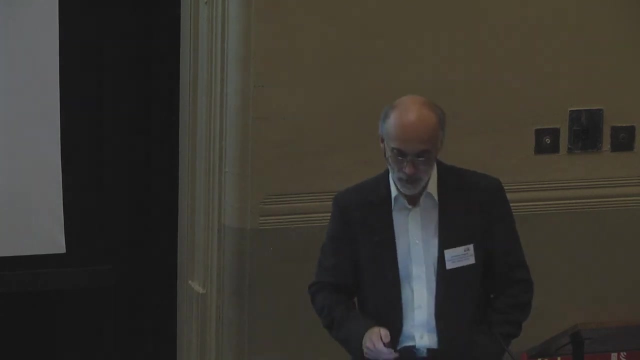 But the fewer square metres they have- especially sensitive ones- left to lose And that counteracts the acceleration and you end up with a straighter line And then the rest of the budget can be closed. can be explained by mass loss from the Greenland ice sheet. 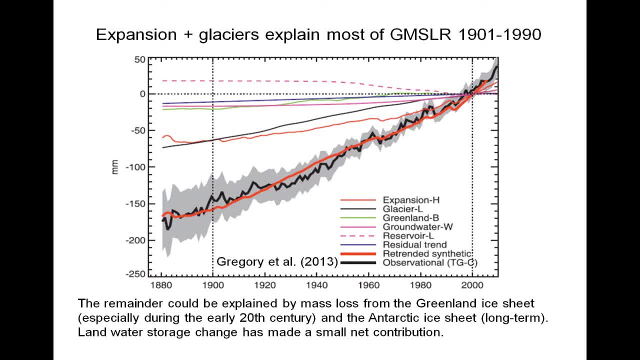 especially during the early 20th century, when models suggest, and data suggests, that because of the warm period, the ice sheet may have lost mass at a greater rate. And the Antarctic ice sheet which is shown here as a straight line, that's this dark blue one here. 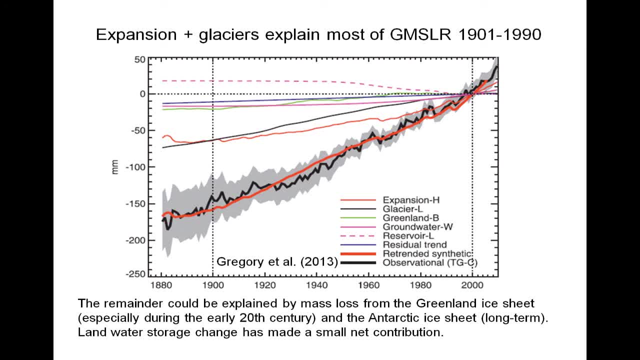 effectively just to close the budget. but to close the budget requires only, in this case, 0.1 millimetres a year, which is consistent with a long-term adjustment of the Antarctic ice sheet to the end of the last glacial, as Jonathan mentioned. 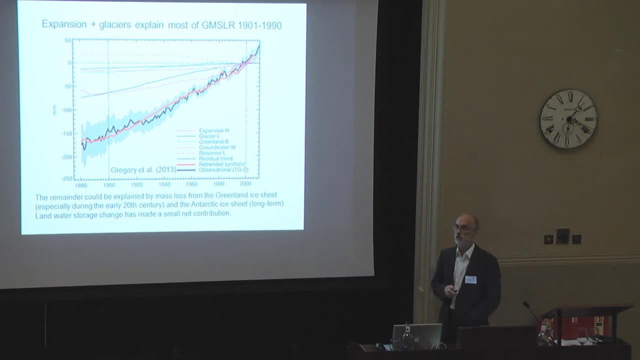 and is not inconsistent with the proxy evidence of sea level change over the last couple of thousand years, But it permits a small contribution like that. There's also a net contribution from land water storage, which is these two lines. The solid one is the groundwater mining term, which has increased markedly recently. 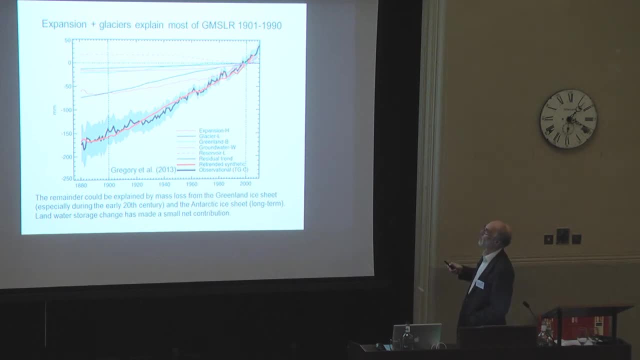 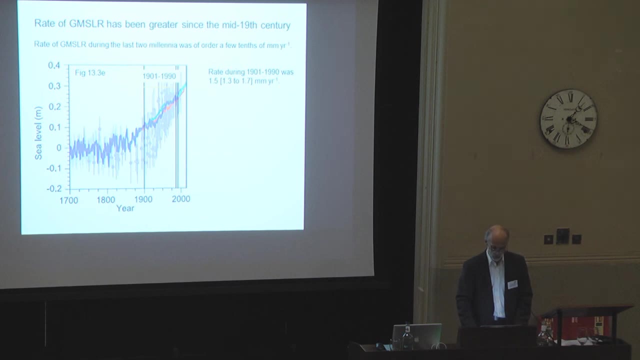 And the dashed purple line is a negative term due to reservoir impoundment, And their net effect is rather small during the 20th century. And then when we turn to the recent years. Annie has already discussed this budget, so I needn't do so. 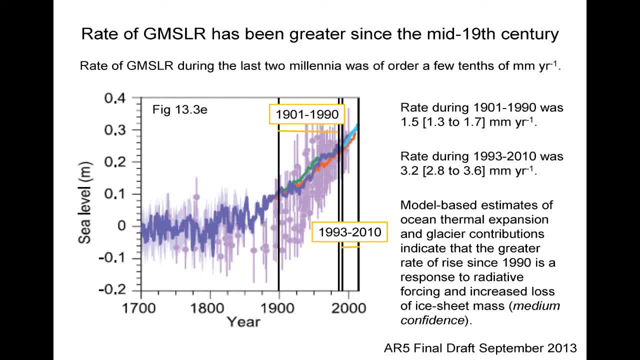 We find that there is a greater rate of sea level rise, and model-based estimates suggest that this greater rate is at least partly forced because of the greater thermal expansion and glacier mass loss. But there is also the contribution from the ice sheets which has increased and that may not be anthropogenetically forced. 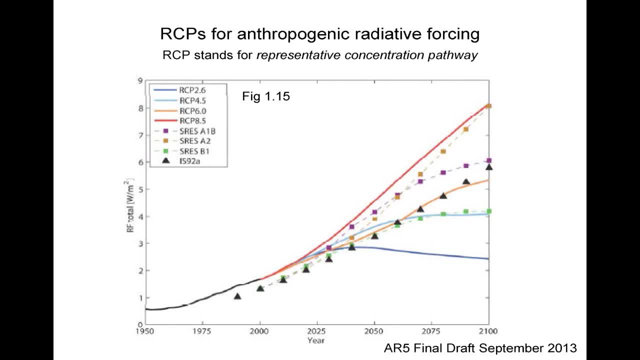 That might be internal variability. So now then, turning to the future, In the AR5, a new set of scenarios were adopted for considering possible futures, And these are more representative concentration pathways, RCPs. So the difference between these and the preceding SRES scenarios that we used in the AR4 and the TAR is that these are principally concentration time series, not emissions time series. 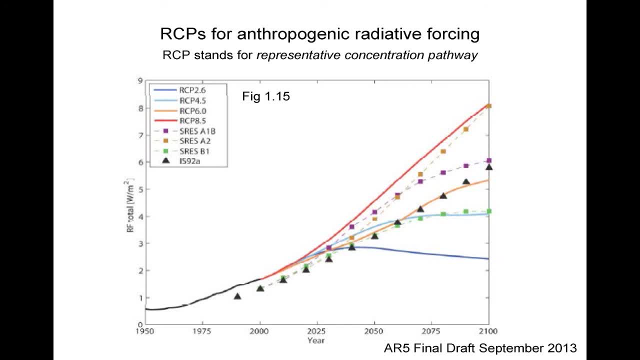 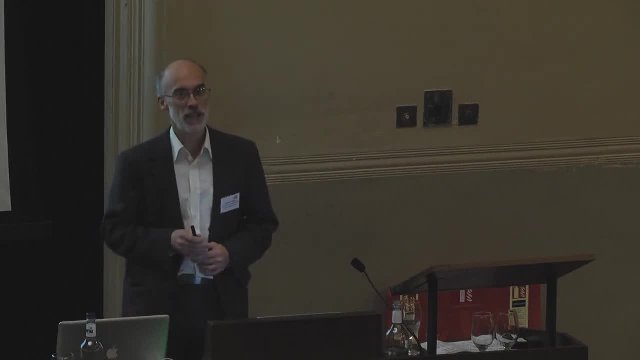 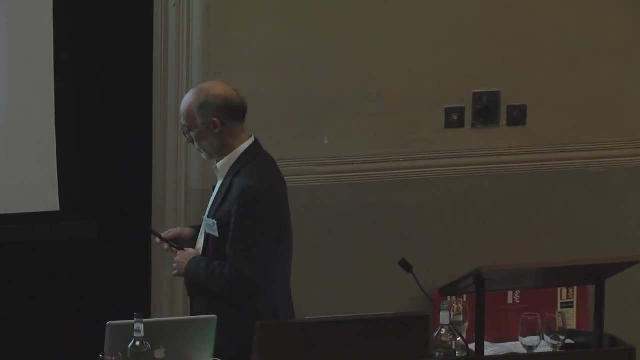 So the job is being addressed backwards with respect to previous assessments. Carbon cycle models are still used, but they are used to work out what are the emissions which would be needed to follow one of these prescribed concentration pathways, And the concentration pathways themselves are input to climate models. 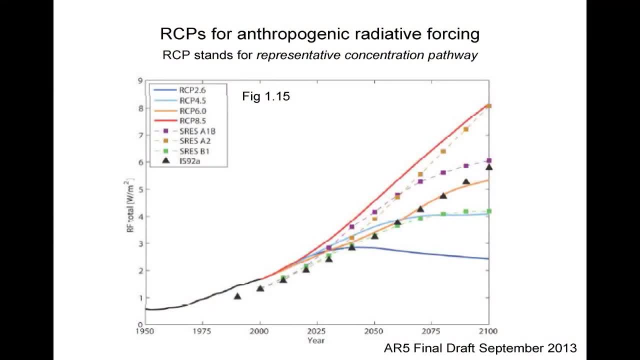 So this graph here compares the rate of forcing of the RCPs- the solid lines- with the SRES scenarios that we used in the AR4. So you see that the scenario of greatest concentration increase- RCP 8.5, is comparable with scenario SRES A2 of the AR4.. 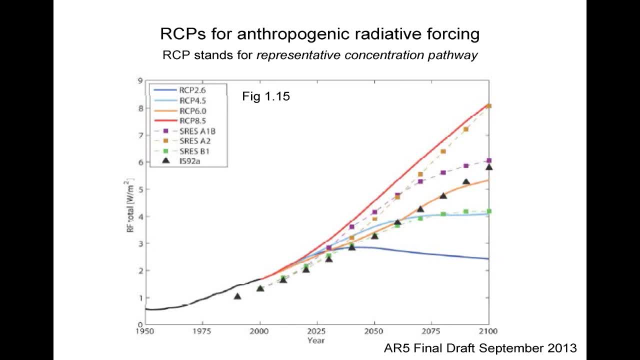 The lowest one: RCP 2.6,. sorry this one. RCP 8.5, is comparable with scenario SRES A2 of the AR4.. The lowest one: RCP 2.6,. sorry this one. RCP 8.5, is comparable with scenario SRES A2 of the AR4.. 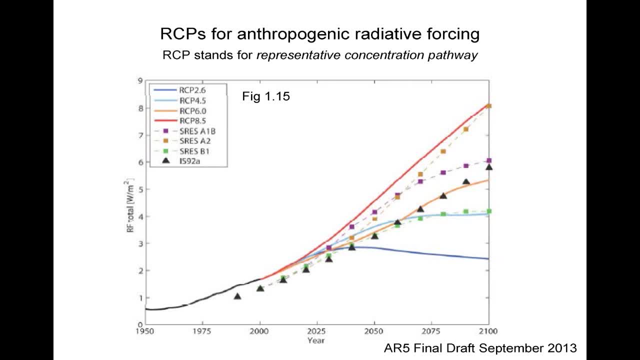 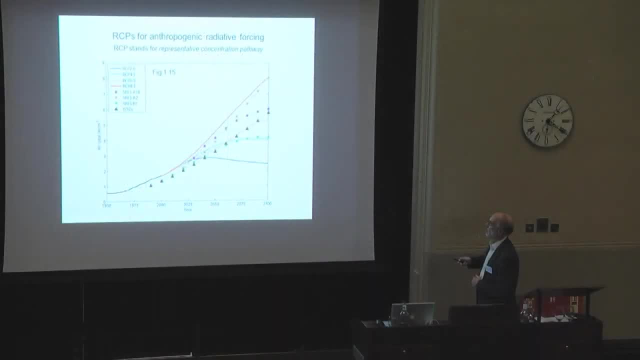 And RCP 2.6 is a much lower scenario than the lowest scenario considered in SRES, that is, SRES B1 here. So this scenario actually has a reduction in radiative forcing by the end of the 20th century, 21st century. 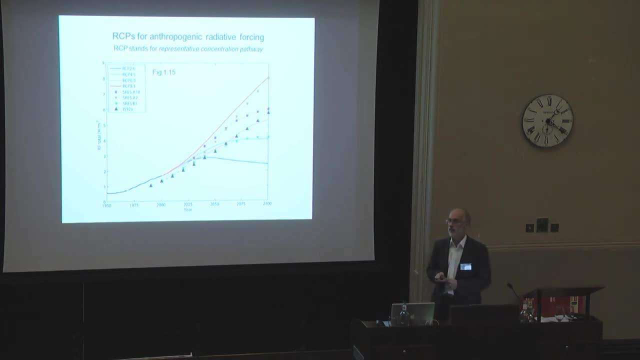 The reason for this is because the RCPs, unlike the SRES scenarios, do explicitly allow for the possibility of policy measures to mitigate climate change, Whereas the SRES scenarios were all non-mitigation scenarios. So RCP 2.6 in particular does imply severe measures taken to limit CO2 emissions. 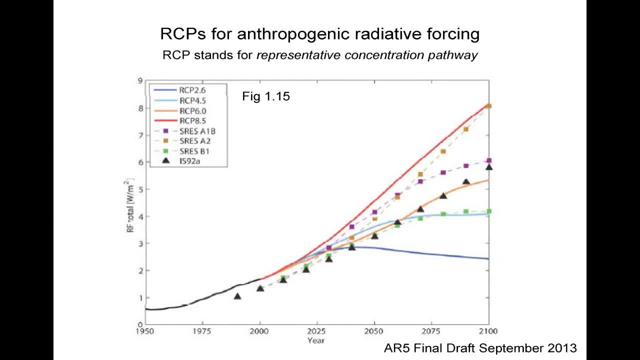 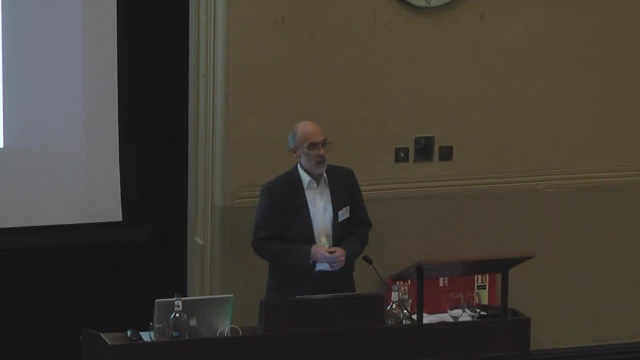 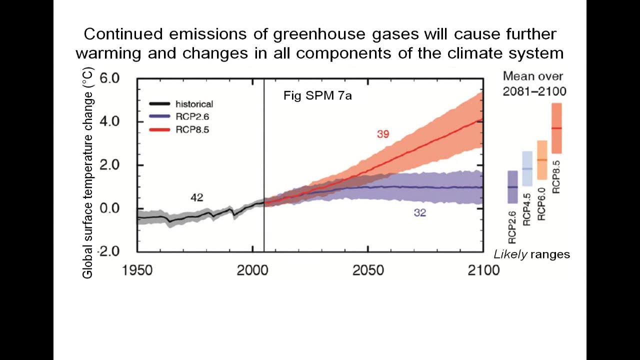 And in fact, to achieve this pathway requires negative emissions in most models in the latter part of this century, That is, taking CO2 out of the atmosphere. Under these scenarios, when they are applied to GCMs, we conclude that continued emissions of greenhouse gases will cause further warming and changes in all components of the climate system. 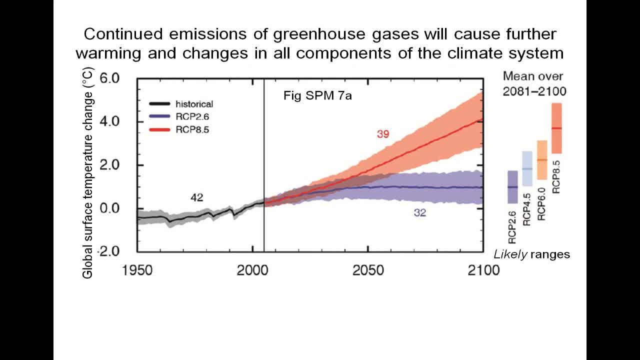 That, of course, is a statement of very high confidence, And the GCM results for global mean temperature change are shown here. The coloured bands are the 5 to 95% range of GCMs And the bars on the right are the likely rain use for 2081 to 2100. 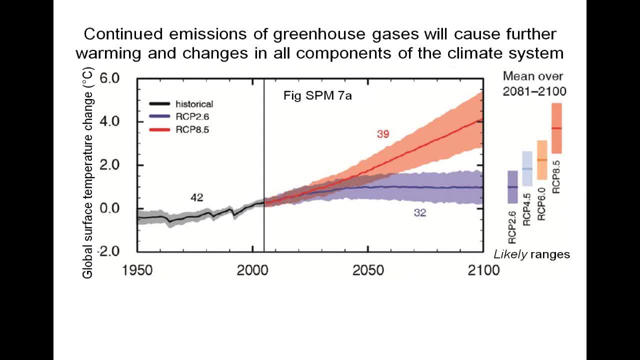 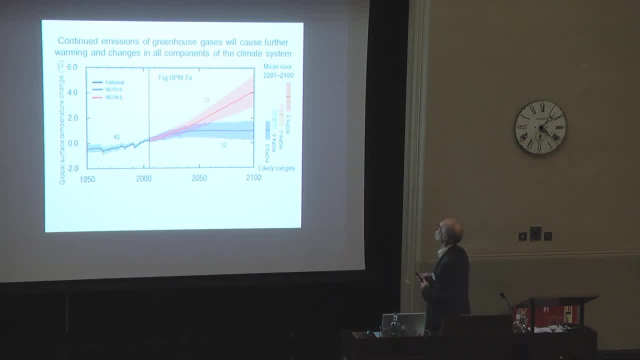 And the likely rain use are in fact the 5 to 95% range of GCMs, But they are interpreted as likely because we don't include all possible uncertainties And they are not very likely rain use but likely rain use And they are not very likely rain use but likely rain use. 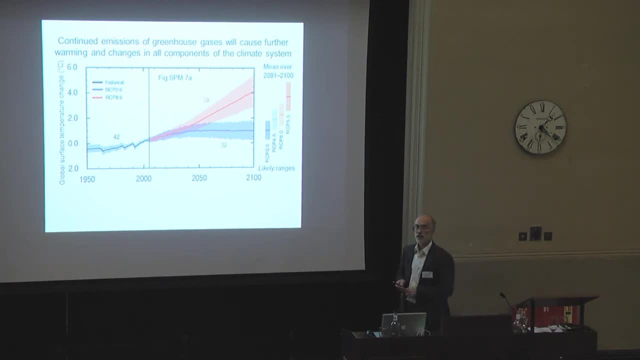 And they are not very likely rain use. but likely rain use Meaning the judgment is: the true answer is: has a two-thirds roughly probability of lying within these bars for a given scenario. So you see, there's a large difference between what you get with RCP 8.5 by the end of the century and what you get with RCP 2.6..